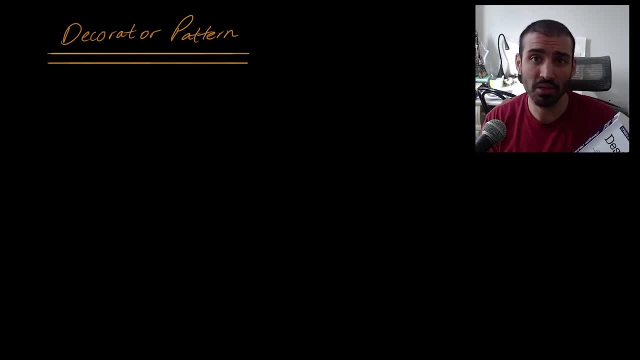 design patterns from this book. In fact, we're going to be doing videos on every single one of the design patterns. The previous ones I've done are on the strategy and observer pattern. I'll put those in the description section below for you to check out. But in this video we're going to be 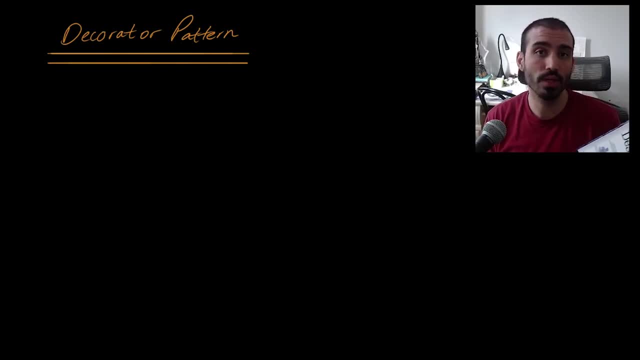 talking about the decorator pattern. So, in terms of the content of the video, I'm going to just define the decorator pattern as per the definition of this book, And then I'm going to talk to you about, conceptually, why it's a useful thing and some of the alternatives that you can use instead. 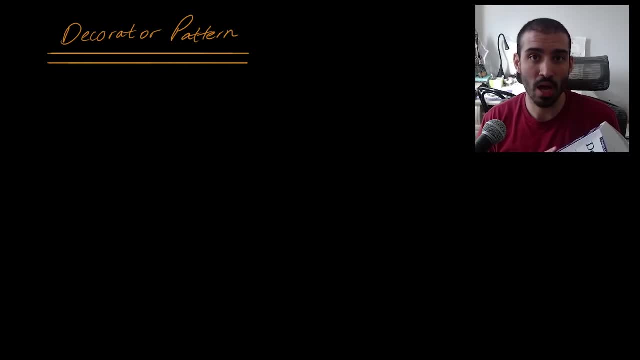 of the decorator pattern. From there I'm going to run through an example On how we would solve a problem if we're not using the decorator pattern, And then from there I'm going to show you comparatively how you would solve the same example using the decorator pattern. 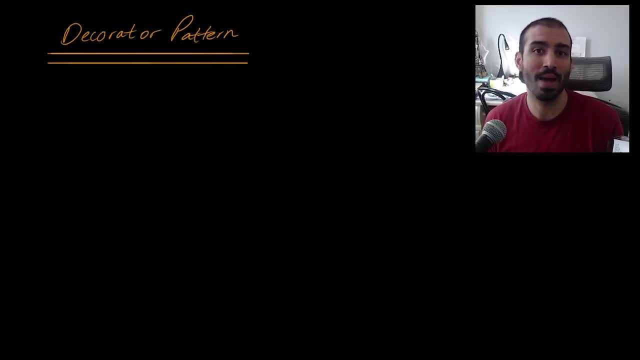 So you get an understanding of how it works in real life and some of the power and advantages that it brings over not using the decorator pattern. So that's what's in store for this video. So let's start out by quickly defining what the decorator pattern is in the context of this book. 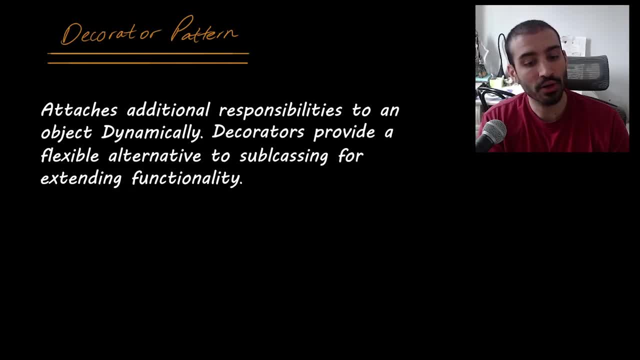 So let's start out by quickly defining what the decorator pattern is in the context of this book. So let's pick this apart a little bit and kind of demonstrate what it actually means. So typically, when you want to add additional functionality to a class, you subclass it. 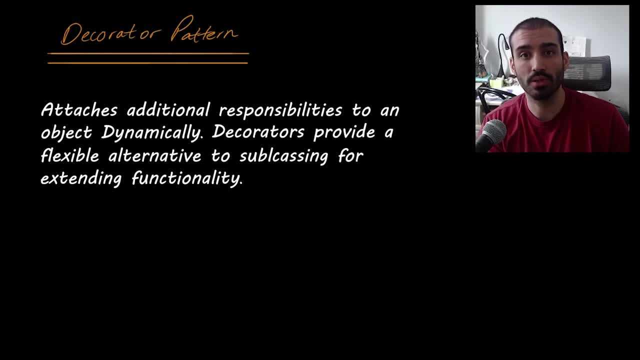 You just extend that class and override some of the functionality that was defined by the parent class. A classic example if you're learning OOP, object oriented programming, is: typically you have an animal or a crop class, which is the super class, and then you have a dog class which is a subclass. 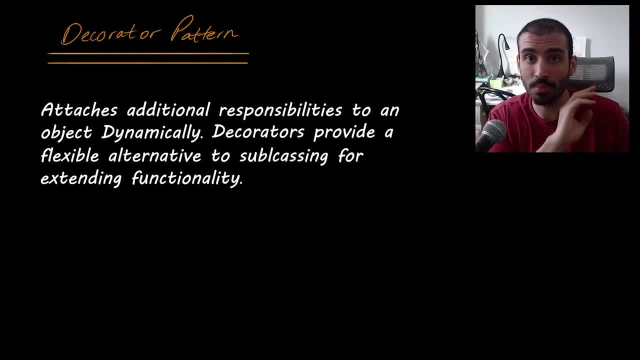 of the animal. and then you know you have a speak method on the parent class and you override that in the dog class. so when the dog speaks it barks, whereas if you have a cat subclass, when the cat speaks it meows. this is typically how you would do subclassing in terms of adding additional functionality and 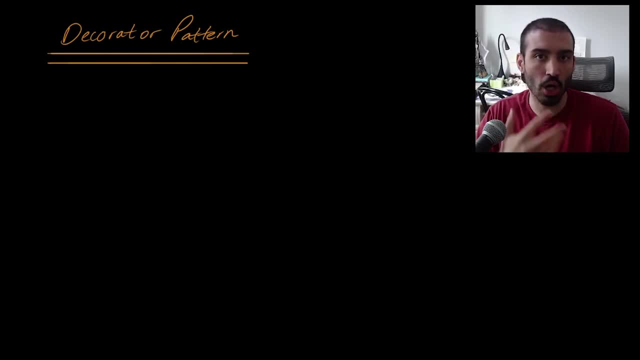 where the decorator pattern is different is that it relies more on composition as opposed to using inheritance, like we saw here- and I'm gonna get into more on like how composition works throughout the remainder of the video- but the main idea, the main takeaway of the decorator pattern- kind of my TLDR for this thing- 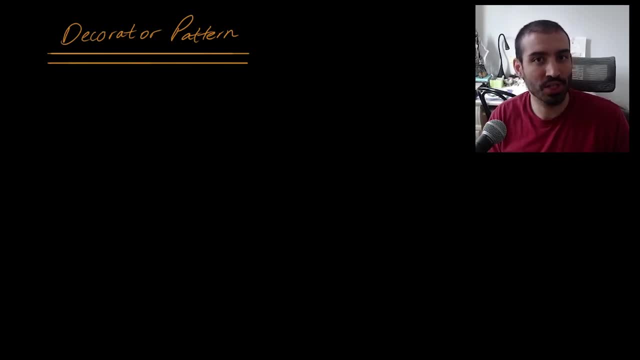 is that, by using the decorator pattern, you can impersonate a class and add additional functionality to it without any of the users of that class actually knowing that it's any different than the real original class. that may be a little bit confusing for you, but we're gonna go through an example shortly and just kind. 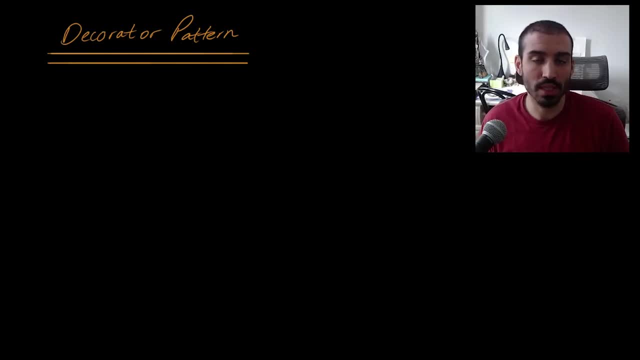 of demonstrate that a little bit more. Now, a common place where you'll see the decorator pattern out in the wild is the javaioinputString class. so if you're interested in seeing an example as it relates to the Java SDK, go and check that out. you can see a whole bunch of 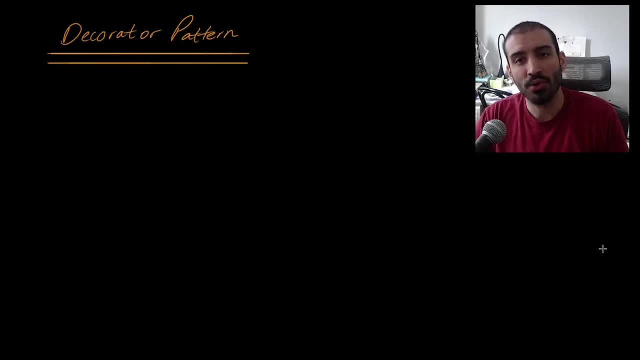 different examples of it. So now I want to move into kind of talking about how you would solve a problem if you're not using the decorator pattern. and the theme that we're going to use in this video is the idea that we're trying to build a system to compute the cost of beverages- for a coffee drink, So we're 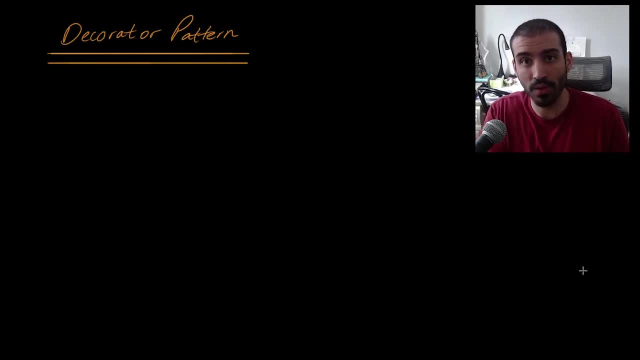 going to start with a coffee shop. Okay, so we have a coffee beverage, we have different types of beverages. there can be, you know, dark roasts, light roasts, espressos, lattes, all sorts of stuff like that. These all have different costs. 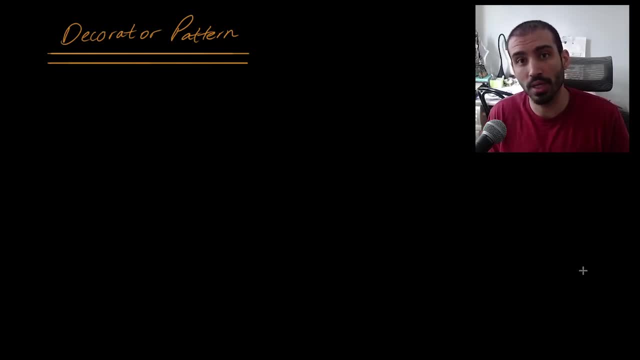 associated with them. and then you can have different condiments or different things that you add to the coffee. that can make it cost even more. So things like cream, things like almond milk, things like sugar, all those kinds of things that you would typically add to a coffee. So let's kind of diagram this out. 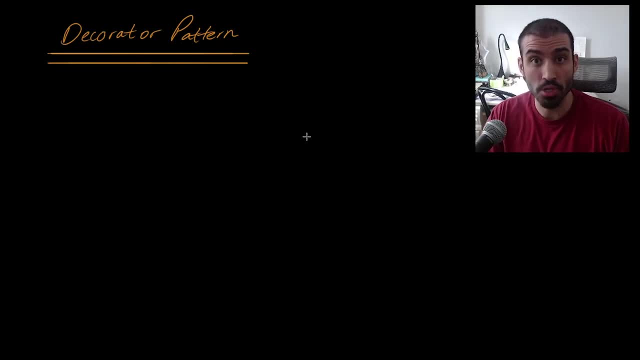 a little bit. I'm just going to kind of do a little rough draft of how this works out if we're not using the decorator pattern. So just reiterating this is not using the decorator pattern in this example I'm about to draw out. 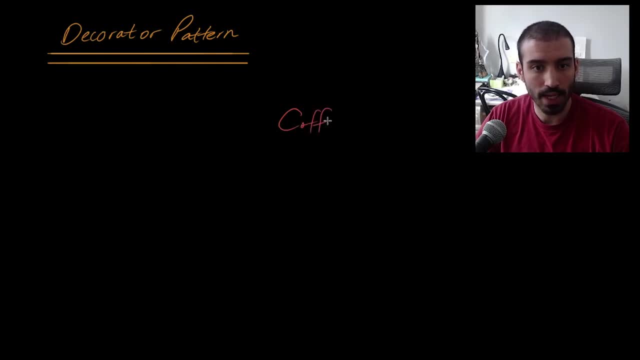 Okay, so let's assume that we have a coffee class here and the coffee class super type has two main attributes: It has the cost of the coffee and it has the description of the coffee in terms of what it is. Now, if we want to add different beverages now like this, is the super type right? we don't really. 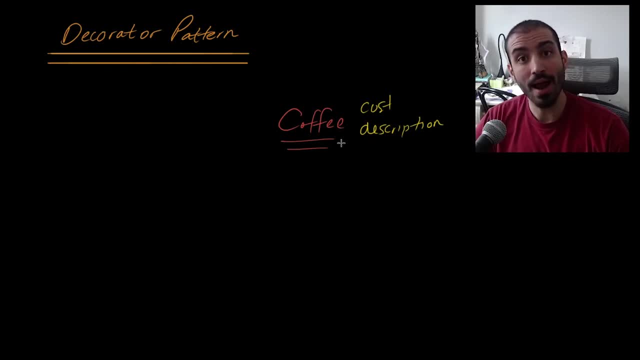 have a concrete implementation of coffee For every beverage that we have on our menu, whether that be espresso, dark roast, light roast latte, anything that we can think of. we now need to subclass coffee so that we can implement the cost and description function and kind of override that. 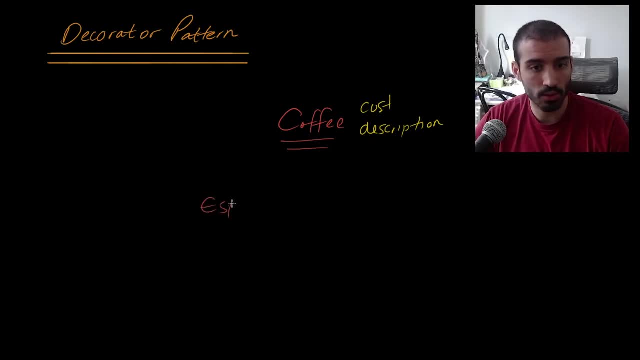 behavior. So what would that look like? So we would have like espresso down here. espresso, we would have like dark roast- I'm just gonna put DR for short and light roast, LR for short. And then what do we need to do now? 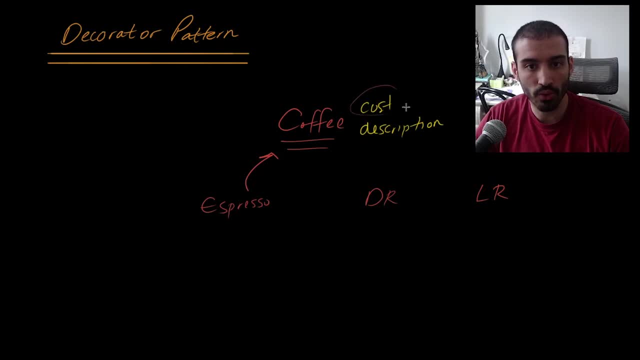 Well, espresso needs to extend coffee, and then it needs to override the cost and description function. The same thing needs to happen for dark roast, The same thing needs to happen for light roast. So so far this is making sense. There's nothing really too insane about this. 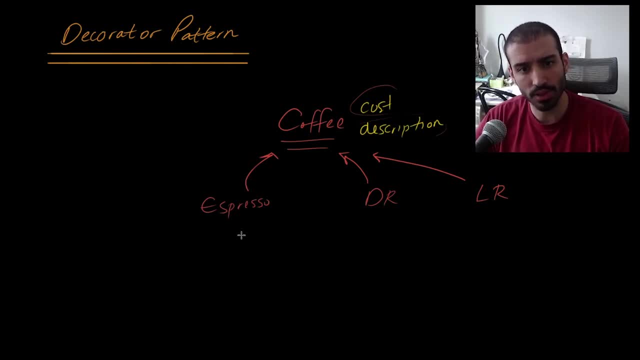 We just have kind of subclass types for each drink, and then they now just need to override the functionality for each of these different attributes. Now where this starts to get a little bit murky is if we introduce another concept, Say we introduce the concept of ingredients. 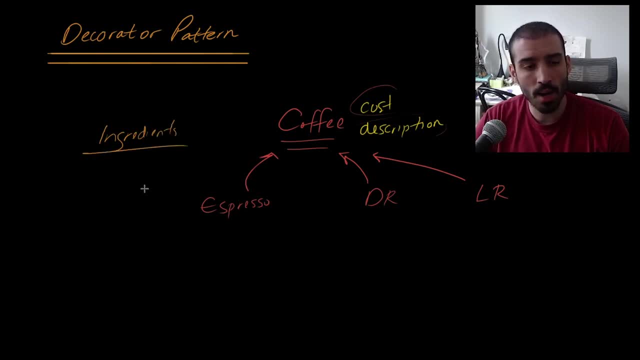 And now we have additional costs based on these ingredients, kind of like I was alluding to before. So maybe we have things like cream that costs I don't know some amount, milk and sugar. You know, these things don't typically cost anything. 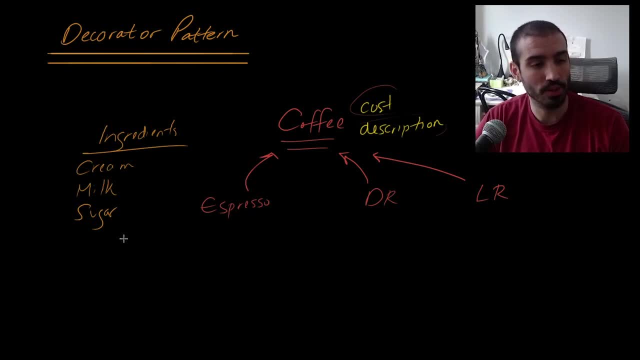 when you go into a coffee shop, but maybe some of them in the more gourmet ones do. But you know, you can quickly extrapolate this. if you have more expensive ingredients that actually do cost a lot. You can easily see how this would be applicable. 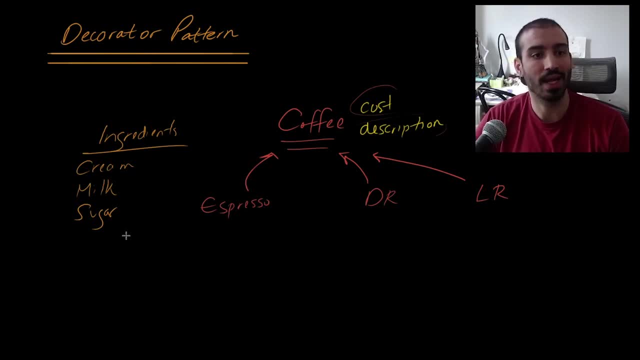 Things like I don't know, like almond milk or like agave or any of the fancy things that people put in their coffee drinks these days. So the question is now: how do we incorporate this ingredients concept into this relationship, So something that kind of sticks out on my head? 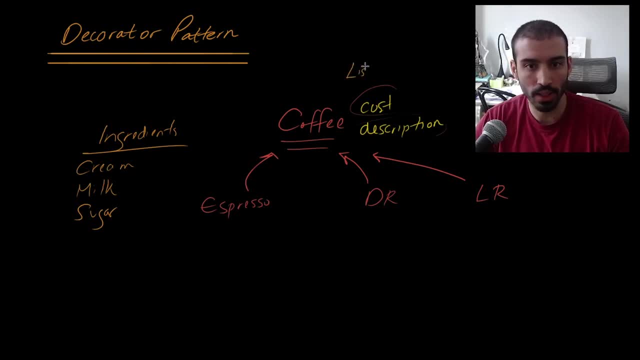 is that you would introduce a concept of like ingredients, So like a list of ingredients, Ingredients- Sorry, my writing is a little bit terrible there- And then each of these different types of ingredients- so cream, milk and sugar- would be a different. 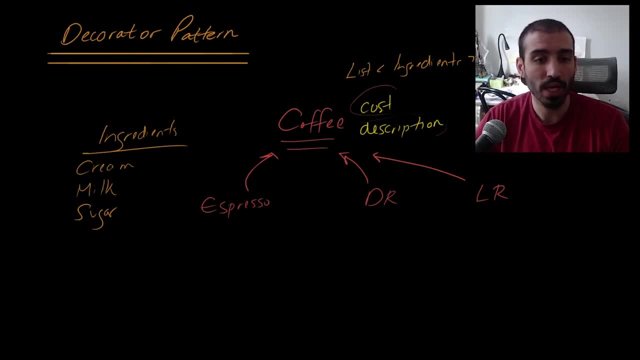 a different implementation. They have a different cost associated with them as well. And then when you're kind of building this espresso object, you add, like you know, 2X sugars, 2X sugars. obviously no milk or cream for espresso. 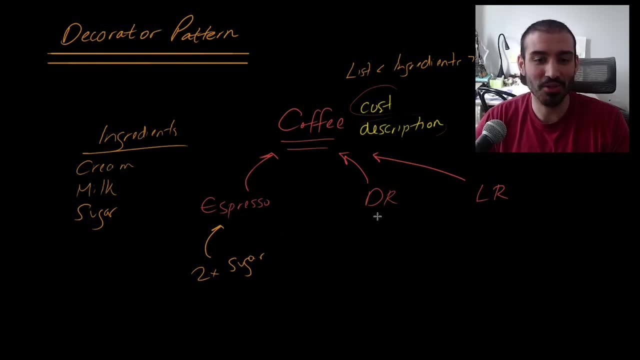 You should never add milk or cream to an espresso. And then in your dark roast you can do things like you know: 2X sugar, 2X sugar, and then maybe like 1X milk, right, And then you can potentially just compute the cost function. 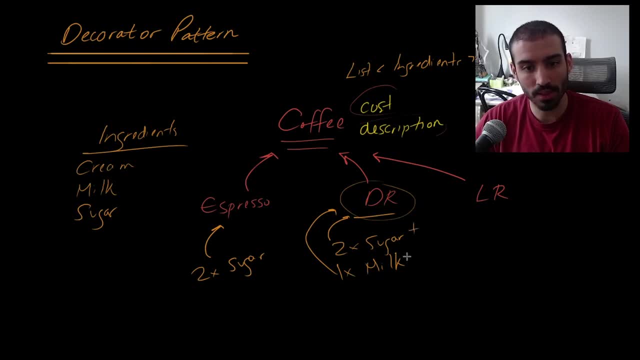 considering the base cost of the dark roast plus the sugar, plus the milk, And then in the end that's what your cost is. So there's nothing wrong with this approach. This is kind of the classic inheritance type of way to do this. 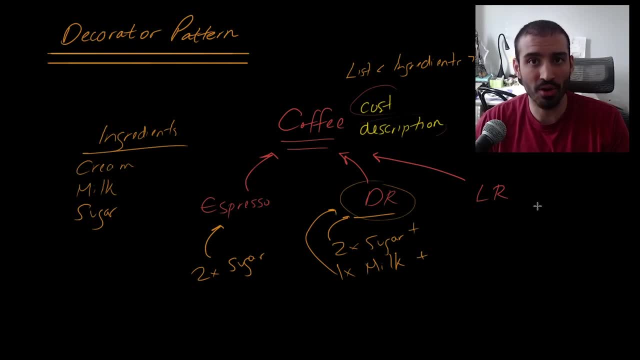 The problem is that you're going to get a class explosion as you add all these different ingredients, add all these different types of beverages. It tends to get a little bit complicated there, but I just want to kind of tell you there's nothing inherently wrong with this. 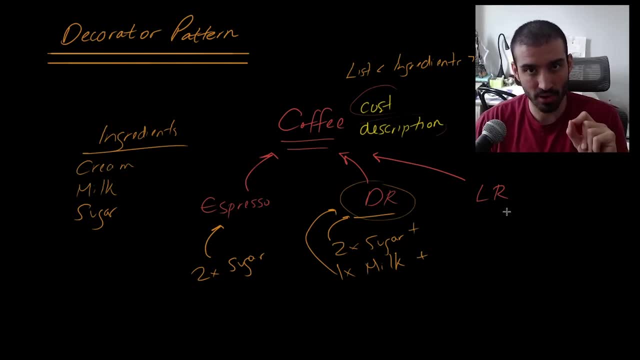 Let's go through. We're going to do the same exercise using the decorator pattern, And where the decorator pattern is different is that we're going to use composition and some clever type matching tricks, using abstract classes in the Java language, to basically impersonate the coffee class. 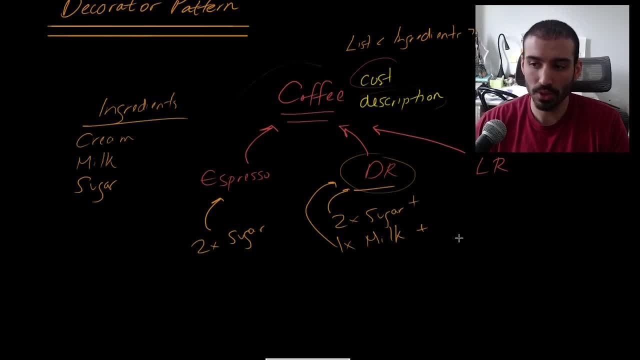 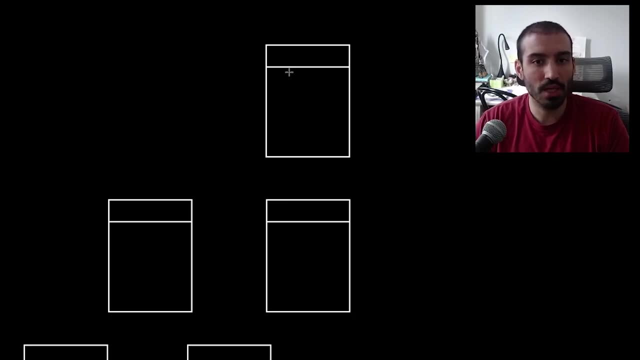 and do this in a slightly different way, And this is going to make sense to you in a second here, So let me just scroll down here. so I have all the class diagrams that I want to draw out, Okay, so just a little bit of a warning here. 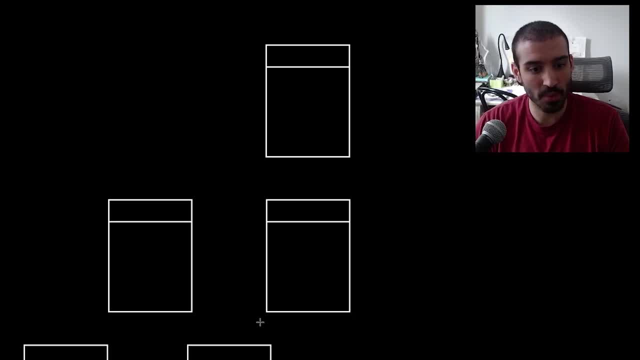 It may be a little bit confusing in the beginning, but I promise you, once you kind of look at this from a big picture perspective, it'll make even more sense when you look at this from the code, because I'm going to walk you through how the code actually is constructed. 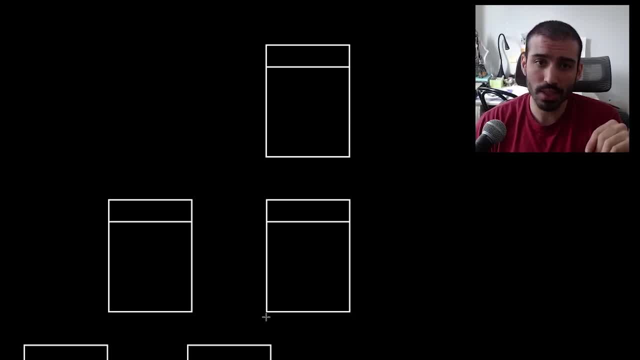 once we're done with constructing these classes. So, using the same example, let's walk through what happens here. So we still have this coffee object, so coffee object And this thing again is going to have still a description. I'm just going to put DESC and cost. 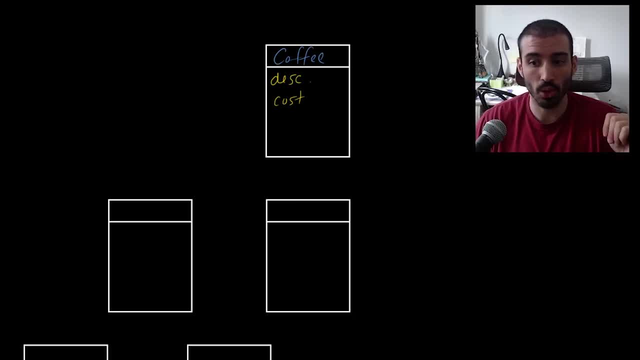 So it's going to have these two attributes and maybe some access or functions that go along with it. Now, in this example, the coffee class is going to be abstract. No one is going to actually be instantiating an instance of this coffee class. 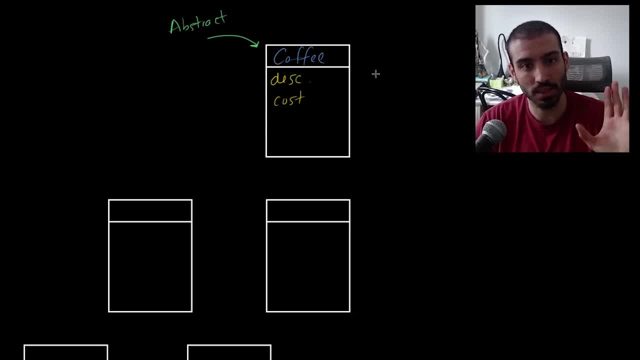 It's just going to kind of be the template in which the subclasses need to use as their specification. So from there we're going to have one subclass And I know I mentioned, like light roast, dark roast, espresso lattes. 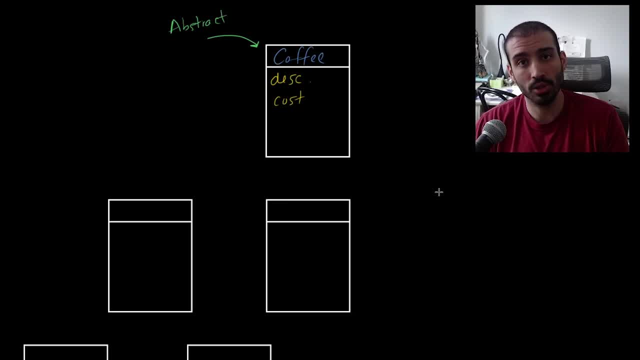 all that kind of stuff in the previous example. I'm just going to simplify it and just use one type of drink, just so you can get the idea. but just know that this applies to all different types of drinks that you may want to add. 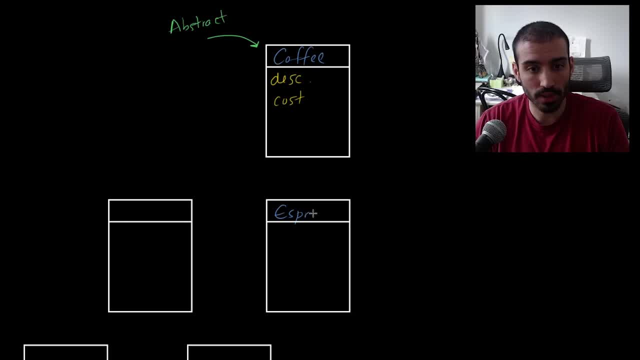 So let's say, now we have this espresso beverage, espresso right, And, like I said, you can have, like dark roast latte, all the different types here if you want. Now the espresso beverage, it has a different base cost. And espresso tends to be a more expensive drink. so it has a different base cost because it requires a little bit more manual work, requires espresso beans, everything that goes into it, So its cost is going to be different. Let's say the espresso base cost is $1.99.. 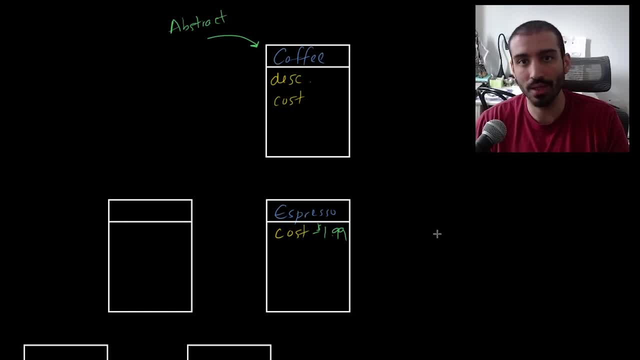 That's what an espresso costs. A latte can be $2.50 or $3.. You can add anything to any different types that you want, but the espresso's cost is $1.99 in this example, And the espresso is going to implement the coffee abstract class. 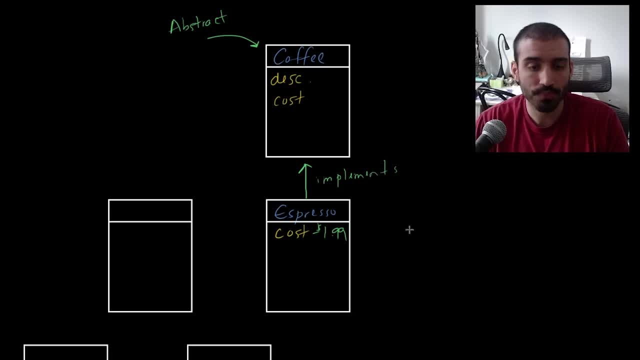 So implements, implements. Okay, that's looking good so far. Now what we're going to do next, which is kind of the interesting part, is that we're going to introduce this concept of the decorator And we're going to say: 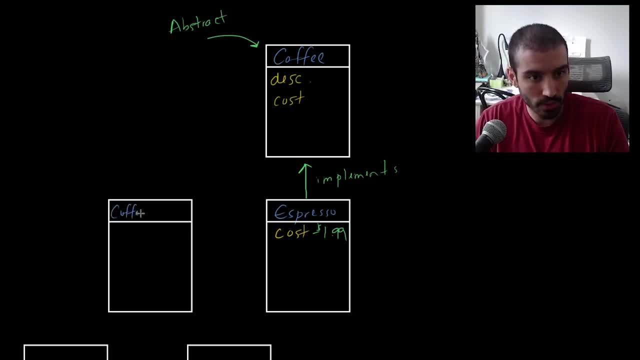 we're going to introduce something called the coffee coffee decorator decorator- Hopefully, don't run out of room. Okay, that's pretty good. And what this class is going to do? it's going to impersonate coffee, So it's actually going to implement coffee. 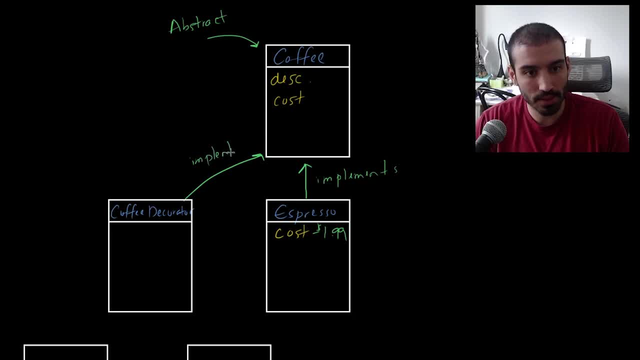 similar to how we did in the espresso Implements, But what it's going to do is allow us to add ingredients dynamically, And that's what these two boxes down at the bottom are going to represent once I fill them out. So the coffee decorator is also going to be abstract. 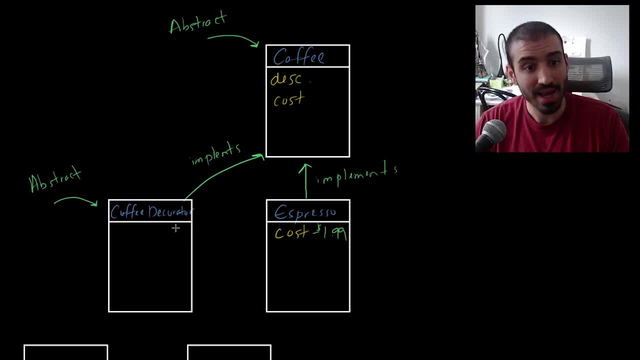 So we're never going to instantiate an instance of coffee decorator. However you can tell like, since it implements coffee, it matches the same signature right. It is still considered a coffee object, So this thing isn't going to really have any interesting properties. 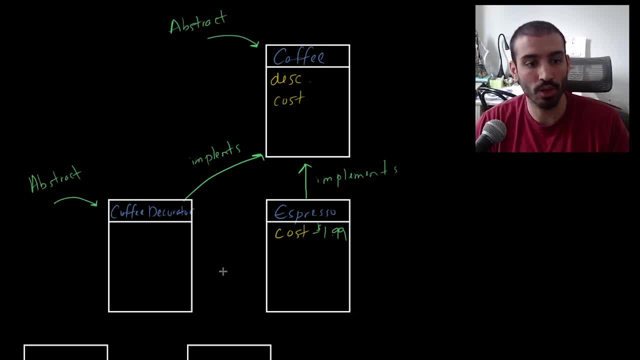 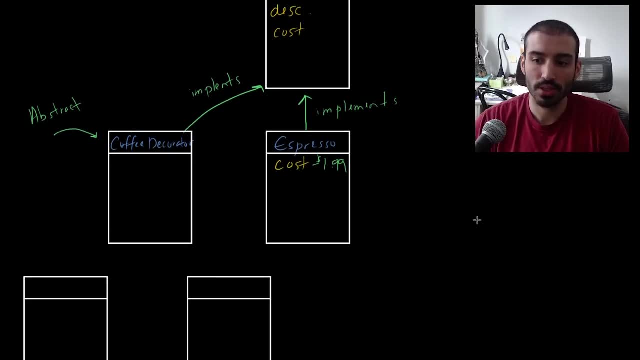 It's just going to be used for some clever type matching magic that we're going to do in the actual implementation. So let's scroll down a little bit and hash out the next two classes here. So from there, we wanted to introduce this concept of ingredients, right? 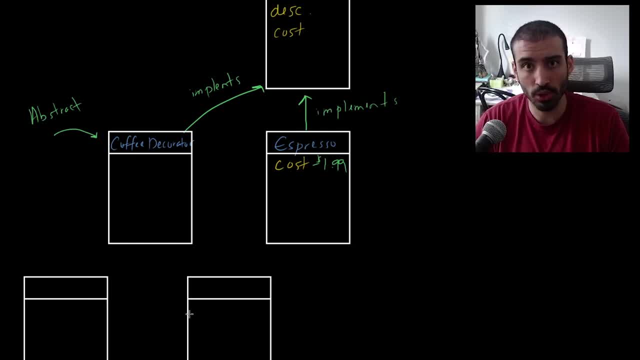 So let's say that these two boxes here are going to correspond to the two ingredients that we're going to use in this example. So we're going to create a class called with milk, with milk, or you can even just call this milk if you want. 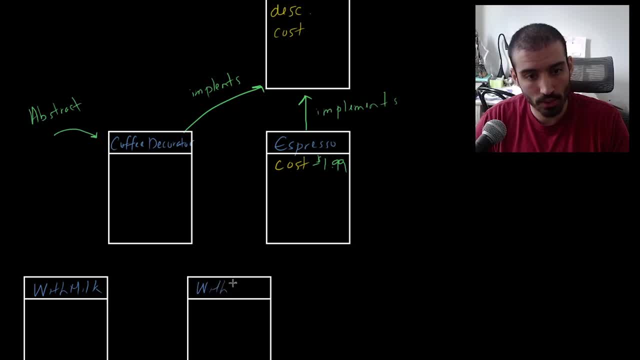 And then we're going to say: with sugar, with sugar And for all the ingredients that you have, you can add additional classes here for this as well. And what we're going to do here is we are additionally like milk costs extra. That was a kind of premise, for example. 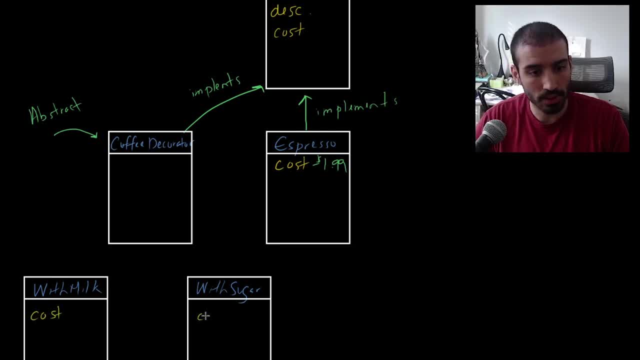 So let's say, the cost of milk and the cost of sugar can be slightly different. So the cost of milk- I don't know like- let's say it's like 50 cents and the cost of sugar is going to be 25 cents, right? 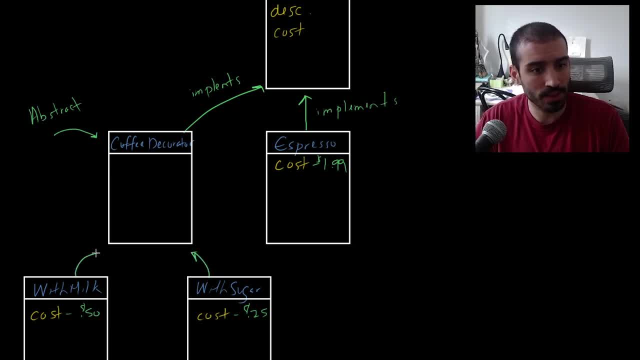 And these two ingredient classes are going to implement the coffee decorator. So the with milk and with sugar are going to implement the coffee decorator and the coffee decorator implements coffee. So with sugar and with milk classes are going to be of type coffee, but through this kind of relationship chain that we built here. 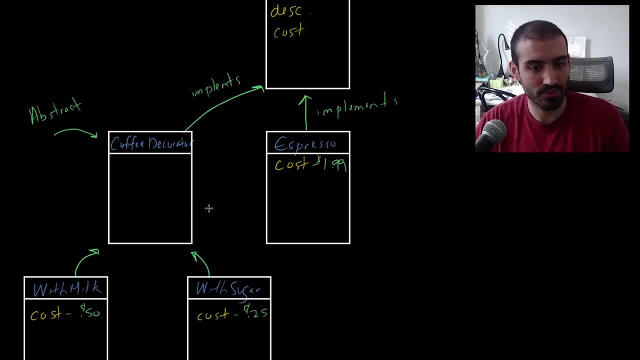 And this is a little bit confusing if you're just looking at this from the kind of class diagram perspective. but I guarantee you this is going to be a little bit more clear once we actually define the classes and show you how it works. But the basic idea here is that now 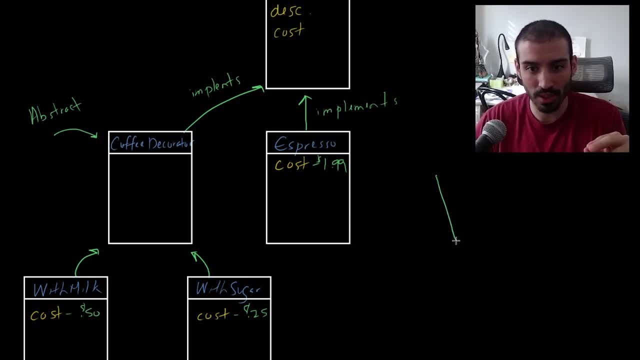 when we construct an instance of our espresso. let me just try to draw out an espresso drink. Wow, that looks terrible, But you know you get the idea. Say this is an espresso Espresso E-S-P-R-E-S-S-O. 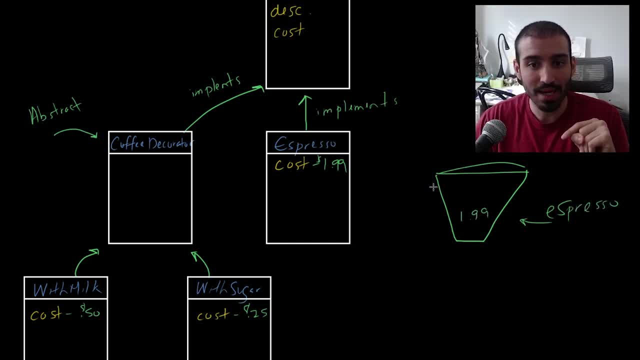 We're going to have a base cost of $9.99, and then we're going to add additional things to it, Things like milk, Milk- And then we're going to add sugar to it- Sugar- And these things are going to cost differently. 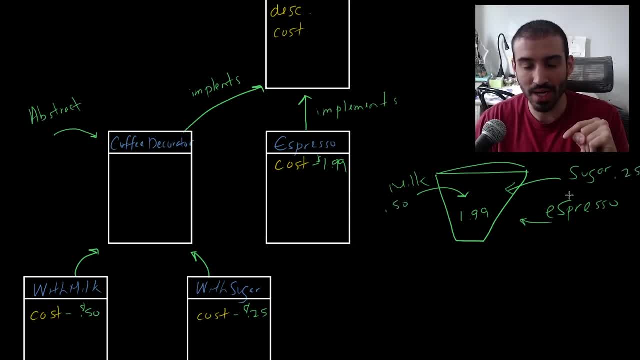 The milk is going to cost 50 cents, The sugar is going to cost 25 cents. But this is all going to be dynamic. We're not hard coding anything here. We're going to give the user the ability to you know. 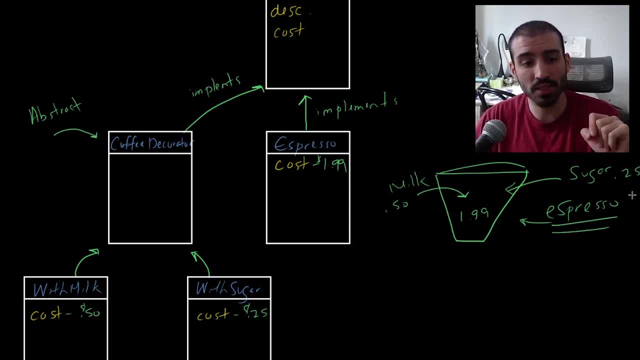 define the base class, sure, but dynamically add all these ingredients And we're going to compute the cost function as the sum of all of the different ingredients and the base espresso in this example. So say, for instance, in this example here: 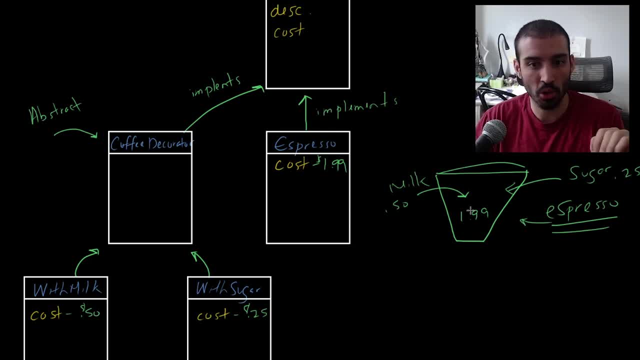 you know you'd have $2 plus 50 cents plus 25 cents, So your total would be 275.. So that's the idea of the decorator pattern. It allows you to do this stuff dynamically and compose your object at runtime. So that's the main idea of the decorator pattern. 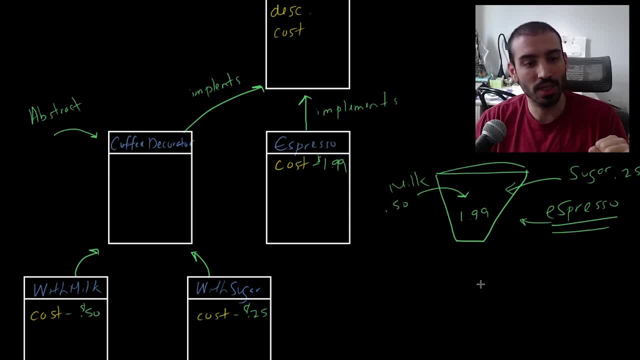 I realize this may have been a little bit confusing if you're just looking at this for the first time, but I promise you, when we jump into the IDE- which I'm going to do right now- this is going to make a lot more sense. 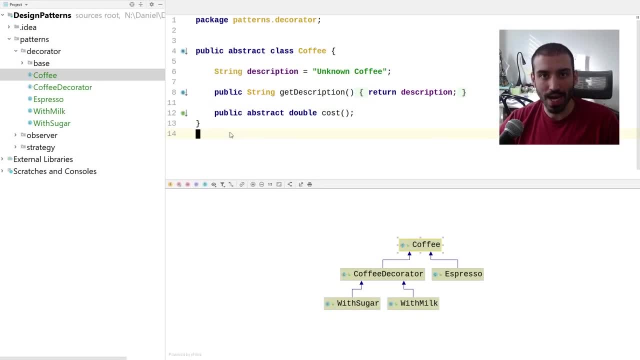 So let's go ahead and do that now, All right guys. so here we are. in my IDE, I took the liberty of creating all the classes that we need for this example and set up the relationships in the way that we just described on the blackboard. 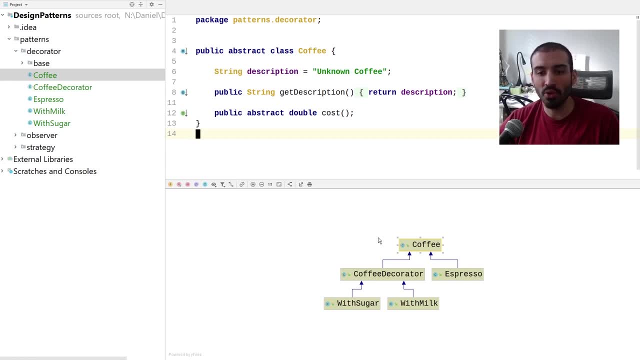 And also use the auto diagram building functionality of the IntelliJ IDE to just generate a class diagram of the classes that we're going to use in this example. So I'm going to leave this section down here up so that you can refer to it and just kind of anchor yourself to what we're talking about. 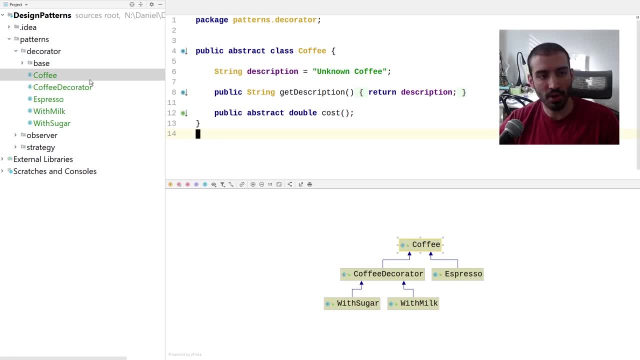 when we go through each of the classes. And just as a reminder, I'm going to leave a link to this code down below so that you can check it out and play with it and just kind of learn by example. So let's run through all the classes that we have here. 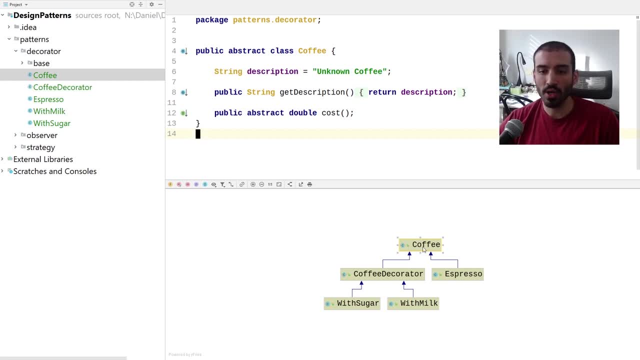 by using this diagram as a reference. So we have coffee at the top And, if you recall, the coffee class is an abstract class. It contains the description and it also defines a cost function, which is abstract, since coffee is abstract in this case. 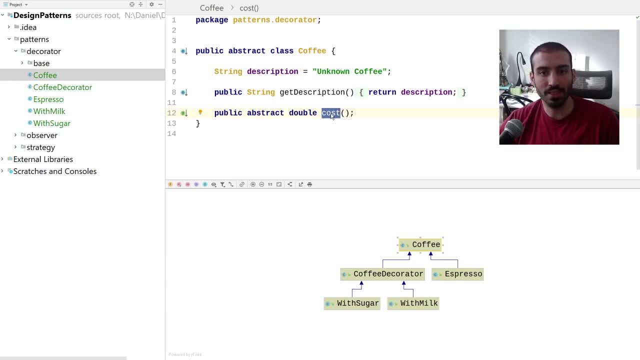 So it is enforcing that all of the subclasses need to define their cost function. So if we go to the espresso class now, which is a subclass of coffee, we see that public class espresso extends coffee and its default constructor just sets the description to espresso, which is good. 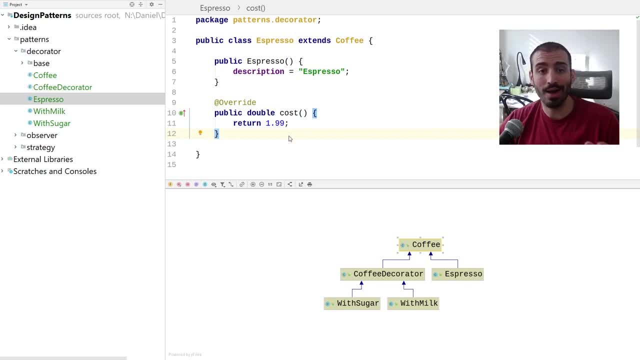 And we said that our cost for an espresso, our base cost at least, is $1.99.. So this is all seeming pretty sane so far. Now I mentioned that the decorator uses kind of a trick in terms of interfaces and type matching so that your ingredients can impersonate objects. 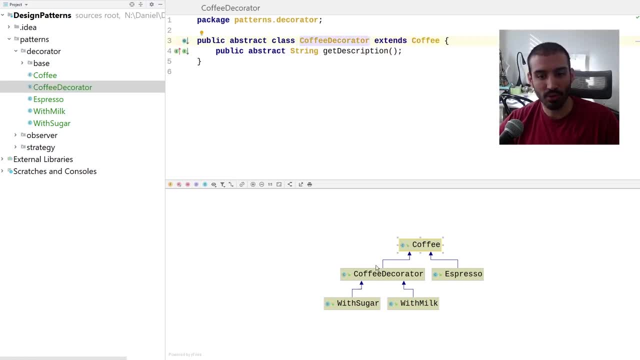 So we see here in the coffee decorator the coffee decorator- and this is kind of where it is positioned in this relationship- it's an abstract class coffee decorator that extends coffee. So coffee decorator is coffee and it's saying that you must override the get description method. 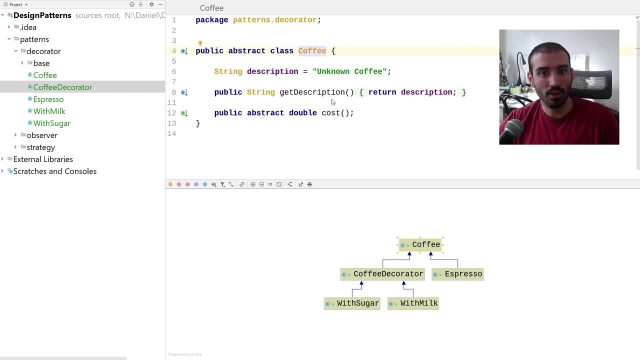 Now remember, in the coffee class we have the abstract cost function, which means that anyone that implements the coffee decorator now needs to implement both the get description method and the cost function. So now let's look at how that works. So we have the coffee decorator. 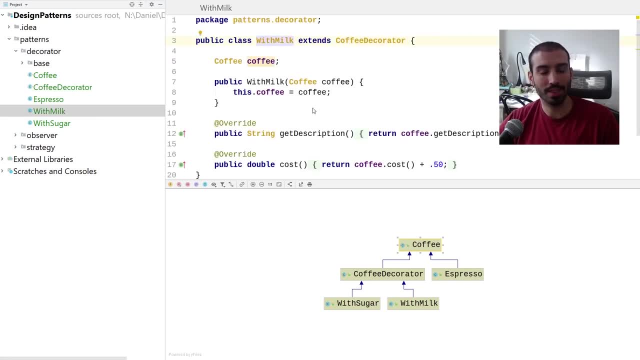 then we have the with sugar and with milk. So with milk, what does this thing do? So this is a little bit interesting. This is really where the magic happens of the decorator pattern. So with this class, we're saying: with milk extends coffee decorator. 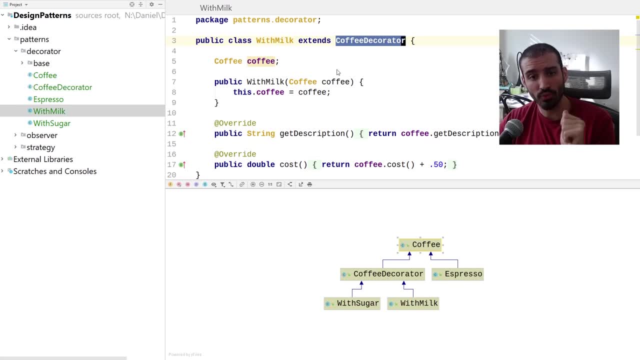 So, right off the bat, we know that we need to override get description and we need to override cost function. That's for sure. And the trick with this class, this subclass that extends the decorator, is that it keeps a reference to the parent coffee object. 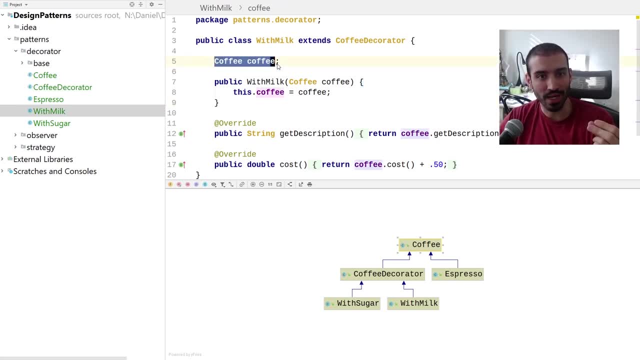 that it was called upon. So we're holding a reference here to a coffee object And we're saying, whenever with milk is called, when the constructor is used, we need to take an already existing coffee object. So you would use espresso in this case. 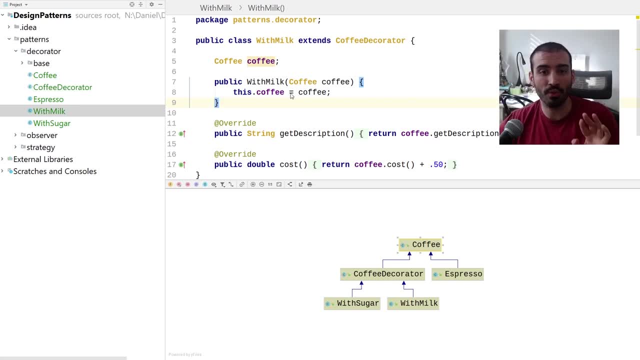 since that is kind of your base object. So now we're holding a reference to it. Now, if you take a look at the implementation of the get description and the cost function, this is where the magic happens. So we say: we return the coffee's get description function. 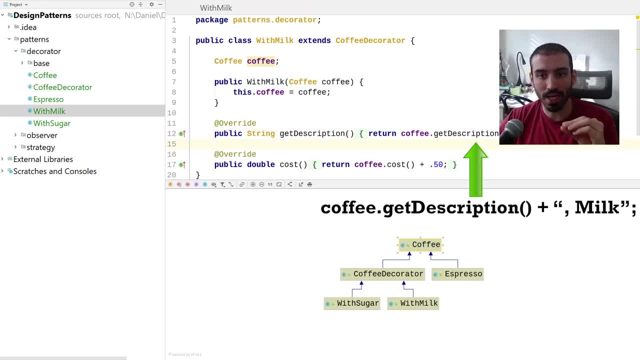 append milk to it in this case. So now we're saying the object now contains an additional property, which is milk, And we're doing something similar with the cost function. You can see down here we're referencing the coffee container instance using its cost function. 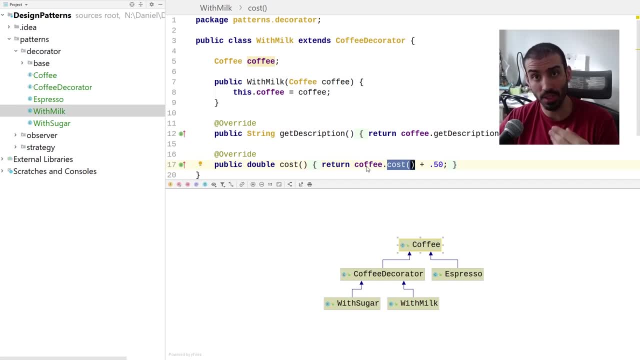 And remember, in this case the coffee's cost is going to be espresso, So it's $1.99.. And then we're adding our own cost, So milk in this case costs 50 cents And you can see if we go over to the sugar class. 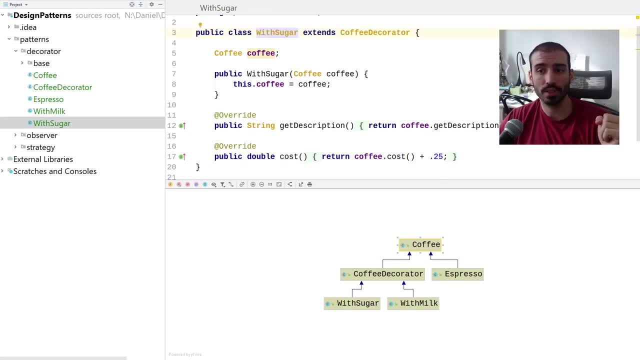 it's basically the exact same thing. The only difference is that we are saying sugar and we are saying our cost is 25 cents. So this is the general layout of the decorator pattern. So this may have been a little bit confusing, but let's actually go to our main class now. 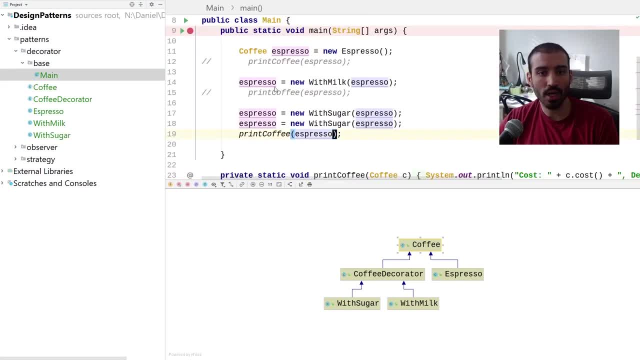 which is our runner, and test this out a little bit. So I have a couple different examples that are laid out for you, So I'm just going to undo some comments so we can work through each of these examples one by one. Actually, let's leave the second one here. 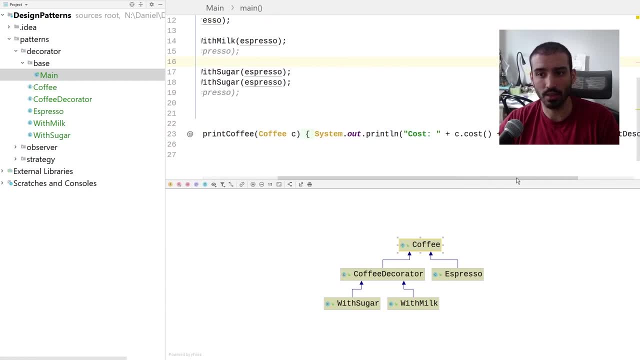 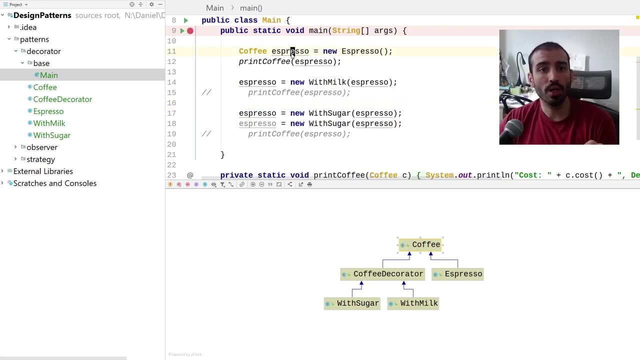 And we just have this helper function down here which just prints out the cost of the beverage and the description, just so you can see what is actually happening. So in this first example we are saying: coffee espresso is new espresso. So what are we expecting to see here? 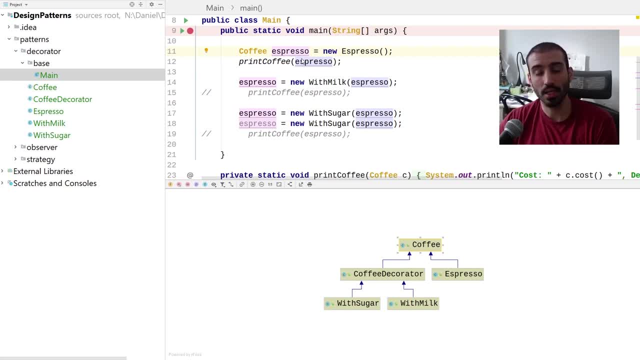 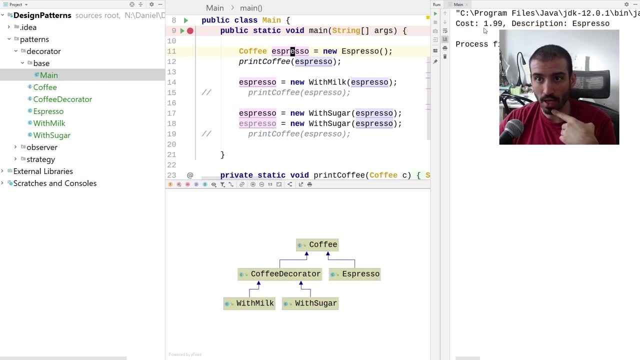 when we print out the coffee's description and cost, Well, we should see $1.99 and it should be espresso. So let's run that now and see how this works. Great, And we can see over here that the cost is $1.99. 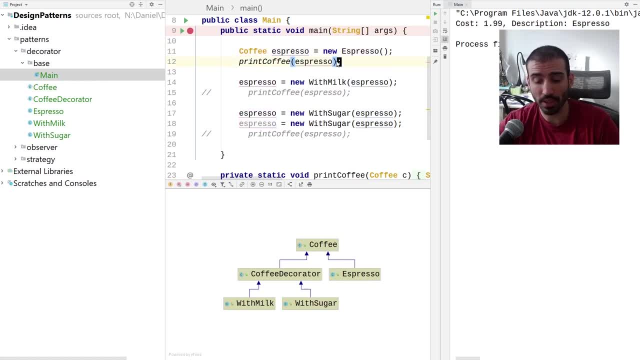 and the description is espresso. Okay, perfect, So the espresso has the right properties associated with it now. So let's take that same espresso object that we just created, and then let's add some milk to it, And then we're going to print the coffee object as well. to see what the cost is and the description says as well. Recall that, if everything worked correctly, milk costs $0.50 and the base cost of the espresso is $1.99.. So it should be $2.49 and we should see in the description. 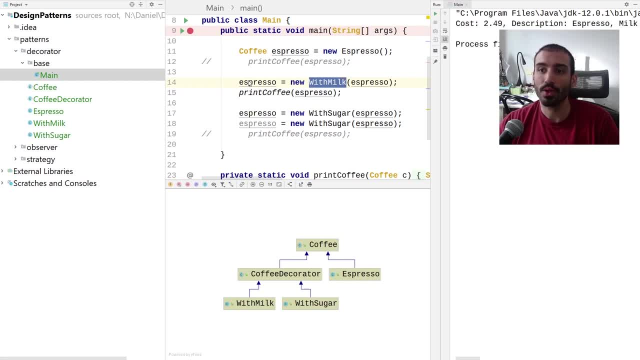 that milk is present as well. Let's give that another run And you can see. the cost is now $2.49 and the description is espresso and milk. Perfect, So everything is working correctly. Now we can do the same thing and add two sets of sugar. 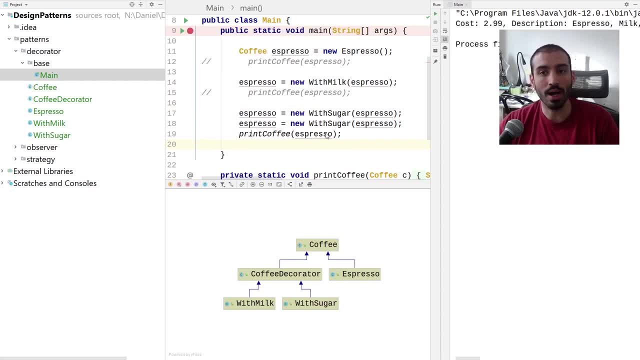 So let's run this again with two sets of sugar. So you should see the cost increment by another $0.50.. So you see, now it's $2.99 and if we scroll over here we can see that now we have two sets of sugar. 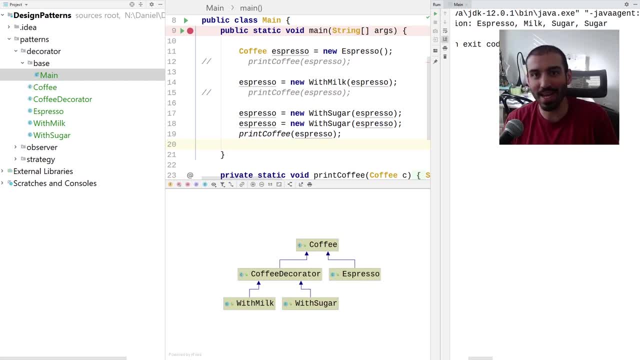 So this is the decorator pattern. This is all there is to it. Again, just to recap on everything that we talked about, the decorator pattern is a pattern that favors composition over inheritance, So you can compose your objects at runtime, as opposed to defining them. 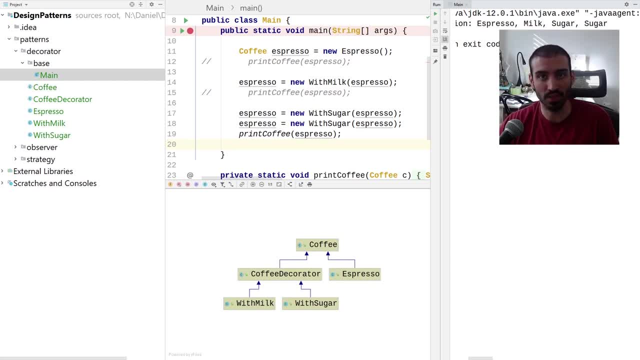 through subclasses, like we saw in the first example at the beginning of this video. If you enjoyed this video, I have other videos on other design patterns from this book. Check out this one on the right here on the strategy pattern, And I'll put a link to where you can get. 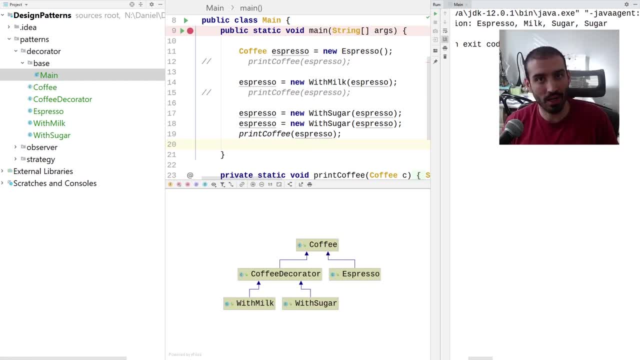 the design patterns book at the bottom of this video. I highly recommend you check it out. It's a really great read And, as always, if you enjoyed this video, please don't forget to like and subscribe. It really helps out the channel. Thanks so much and I'll see you next time. 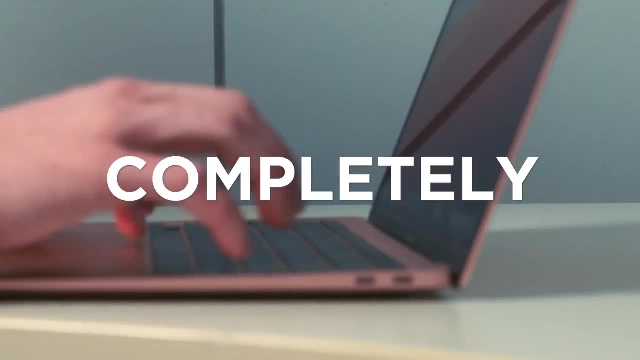 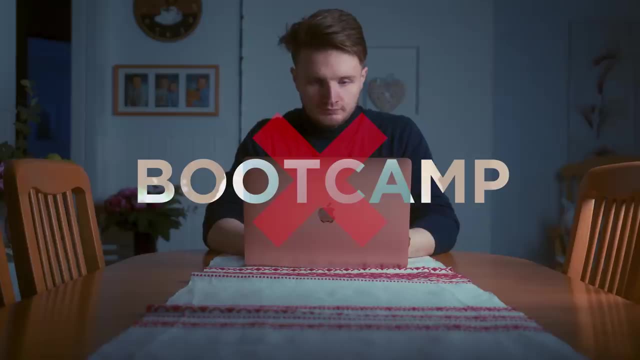 I want to tell you how I learned how to code from completely zero, completely on my own, in just four months, And I even got a job as a software engineer after that. I don't have a computer science degree. I didn't do a bootcamp, In fact, I've never paid for any. 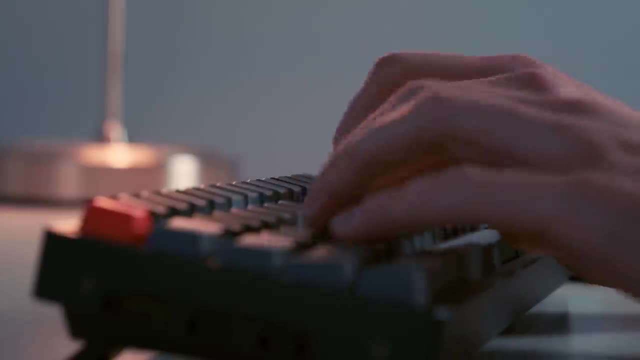 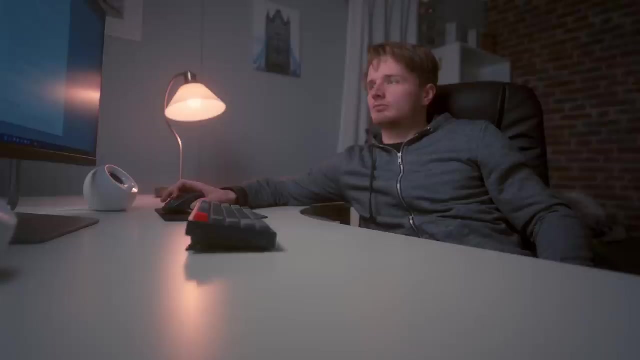 materials that I've used to learn coding, Because in this day and age, coding is a skill that you can learn for completely free on the internet. I am proof of that and in this video I want to tell you how I did it. So just a few months ago I had no idea what.